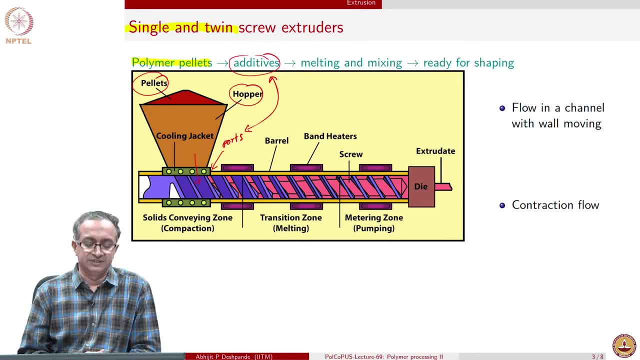 are for stabilization or any other feature that is desired, and if we, let us say, are making a blend, then we will have to have pellets of both of the polymers. If we are making a just one polymer, homo polymer, then we just have a one single polymer. 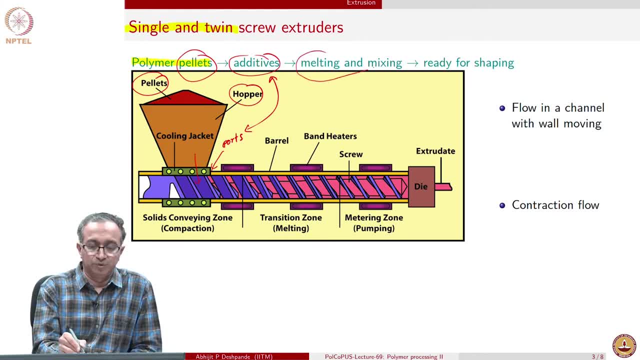 But in both the cases we will have mixing and melting involved, because there are additives and a single polymer or two polymers being mixed, And once melting and mixing has happened, then the overall polymeric system is now ready for shaping and the shaping operation then. 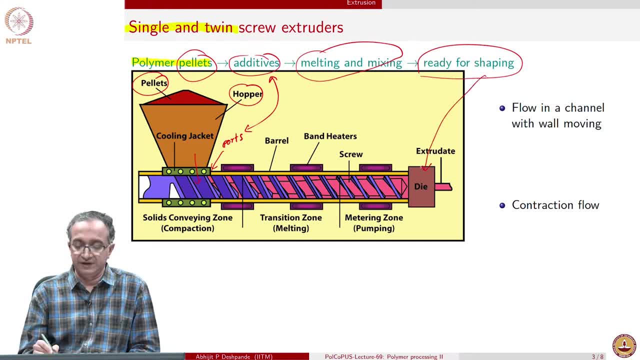 is done using the dye And finally what comes out is called the extrudate. So the process involves. So, if you look at, initially they will be only pellets and that is why it is called a solids conveying zone. In this case, what happens? 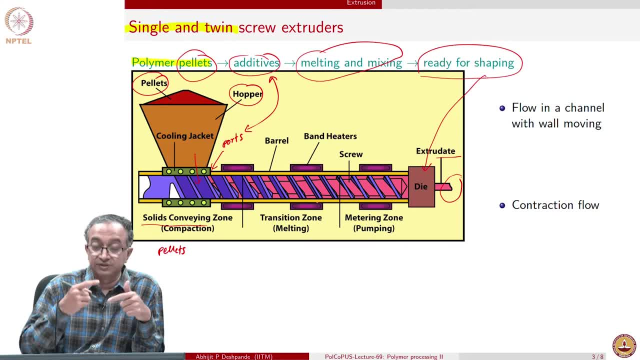 is this screw which is there, is rotating because it is connected to a motor, And so the screw rotation is a very important variable at our disposal in order to optimize this process of melting operation. because faster is the screw rotation, that implies that faster is the delivery of pellets and the compaction that is involved, because we are pushing the 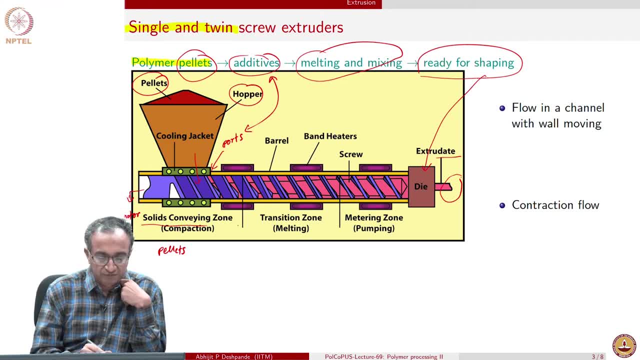 pellets against each other. At the same time, we also will have heating. that is going on because melting is involved. So, given that melting is involved, some amount of heating is done. However, given that this material is getting compacted, given that one layer of fluid is rubbing past the other layer of fluid, or 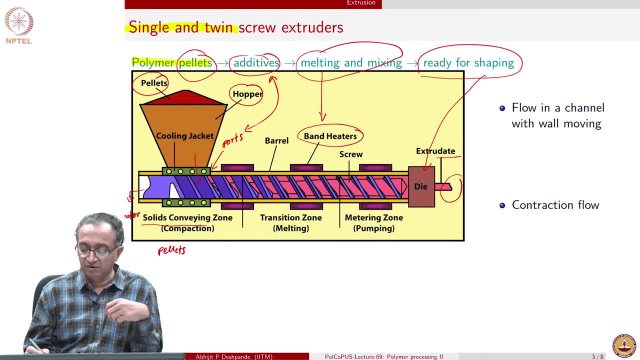 frictional forces, or viscous forces, are involved in all of these polymer processing operations. we have significant amount of viscous dissipation, So some amount of heat is being generated due to the action of flow that we are forcing the polymer to undergo, And so, as material 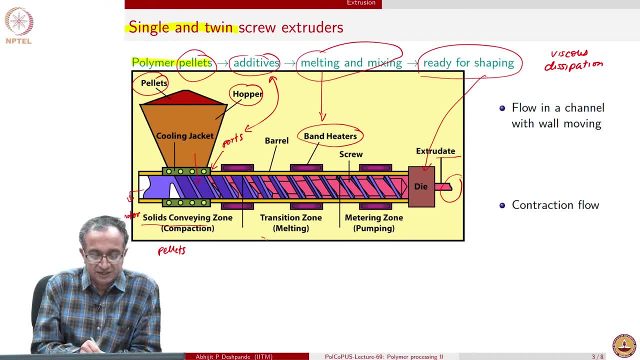 comes proceeds from the polymer. the heat is being generated, So the heat is being released from the polymer. And further we have this transition zone where temperature has increased so that the pellets start melting. And if you look at, let us say we look at this from the side where the between, basically, 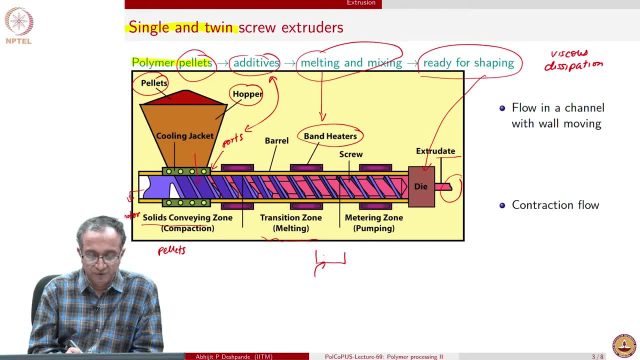 screw. so this screw is rotating And therefore what we will have is the pellets of the polymer. So, initial stages, these pellets will just continue to rotate because the screw is also rotating, But beyond a certain time, once it comes to so, this will be in the solids. 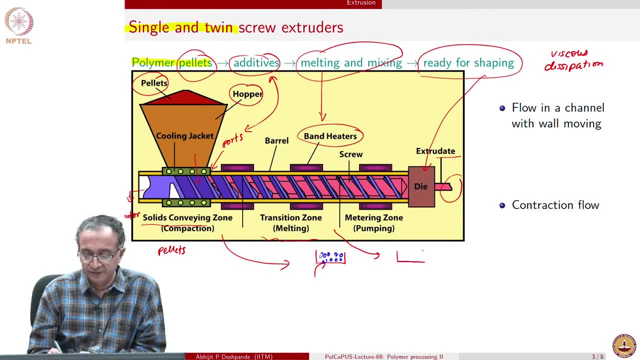 conveying zone. When we come to the transition zone, then what we will have is part of the pellets may still be there and the other part of the screw may already have a melt, And even surrounding each and every pellet. If you look at little more carefully, you may have a pellet. part of it may also be. 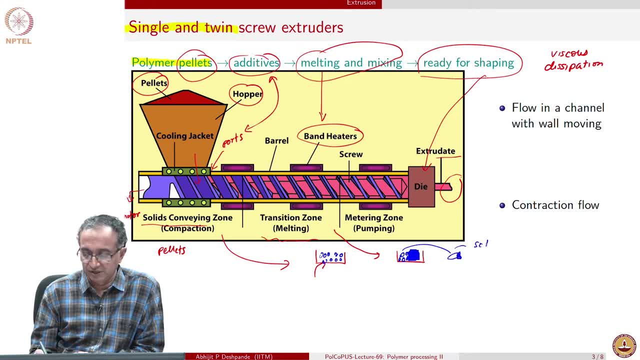 molten. So therefore a solid pellet and a molten pellet. this is at a single pellet level, or we could have melt zone and pellets, So in extruder, by definition, we have this multi-phase flow where there are solid pellets. 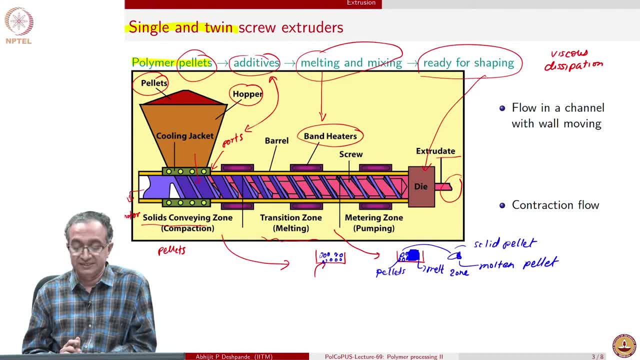 and molten polymeric melts moving simultaneously. And if, let us say, the mixing operation also involves fibers, then you can see that what happens is the polymer surrounding the fiber is going to melt, but the fiber itself may be glass or a natural fiber like cellulose. 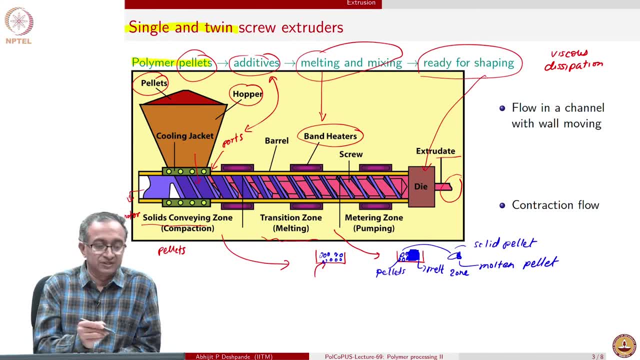 or jute, Then that is not really going to melt, And so what that leads to is basically breakage of fibers, because what you have- and I will draw this picture in a magnified scale- So if you have a pellet, and there is a fiber everywhere in the pellet, and so what happens? 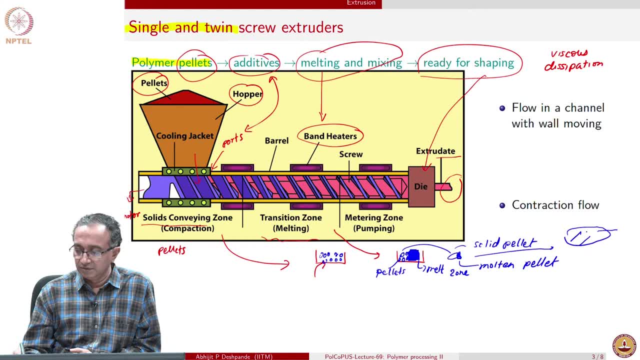 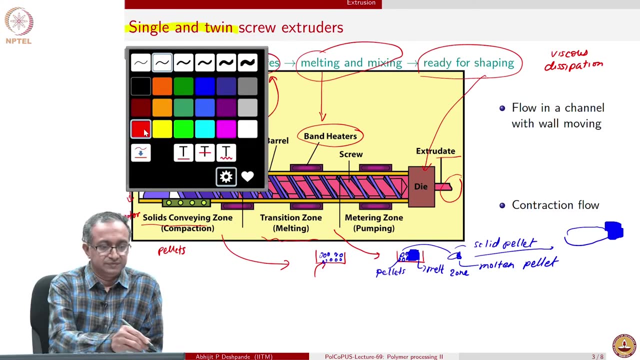 is part of the pellet has molten. I will draw a small rectangle, and so I will have to draw the fibers in a different color so that we can see them. So let us say this is a fiber, and then there are fibers inside. 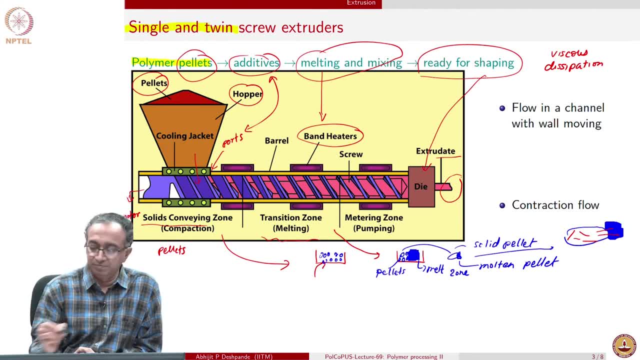 the pellet also. now the molten part can flow, while the solid part, the pellet, embeds the fiber- 1.39. So you can see that this fiber is going to experience a shear force. So this is quite. it is not. it is not a roughители, but it is nothing like the solid part. So there is some kind of a hard edge in it. it is not a hard edge To be able to see that, the solid part. it is not a hard edge, but it is something like the solid part For the most part. you see the solid. 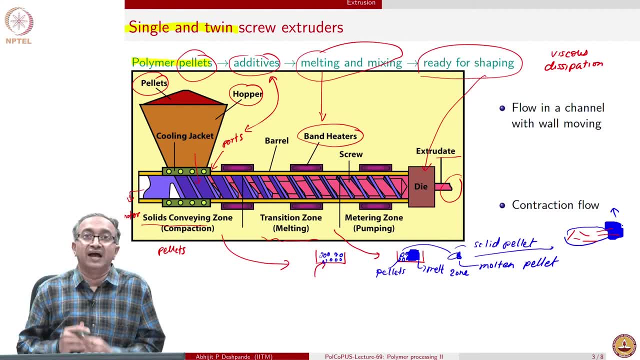 side and the solid part have the different layers. You can see how that this fiber is going to get a lot of friction. You Because the molten fluid is going to move and flow, while the solid pellets cannot move. Of course, the solid pellet can rotate itself, but the rate at which the solid pellet rotates 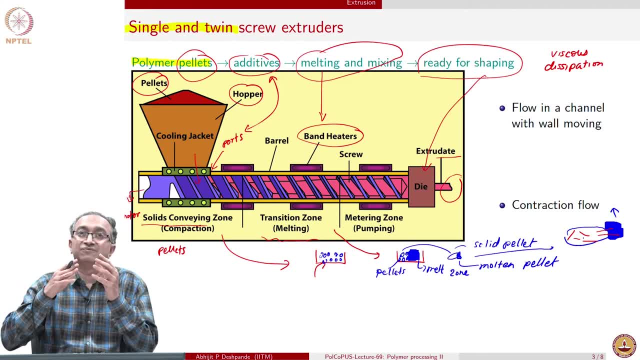 and the rate at which this fluid is moving can be different. and then, therefore, there is a shearing action on the fiber. and what will this lead? to? the breakage of the fiber. So whenever we are making short fiber composites in the pellet, we may have a fiber which is 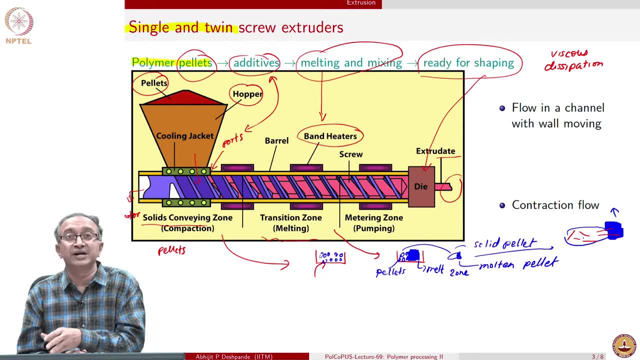 let us say 5 mm, 3 mm long, but in the extrudate the fiber size will be 2 mm or 1 mm, and all of it depends on what happens at a single pellet level and how this melt zone is formed and how does it shear next to the pellet, and so on. 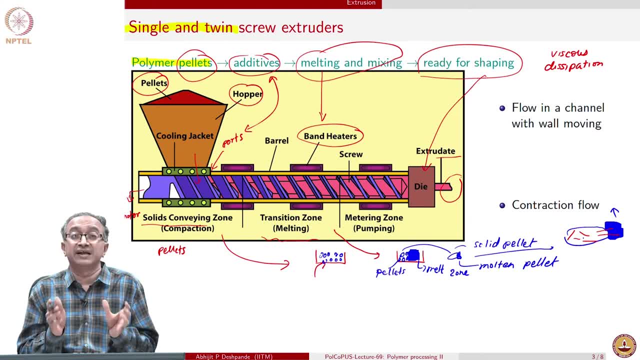 So you can see that, from the importance of analyzing the final product, what happens to each and every section? how are solids conveyed, how do solids start melting, how does the melt flow? This is very important. and then, of course, the final part is the die, and die is necessarily. 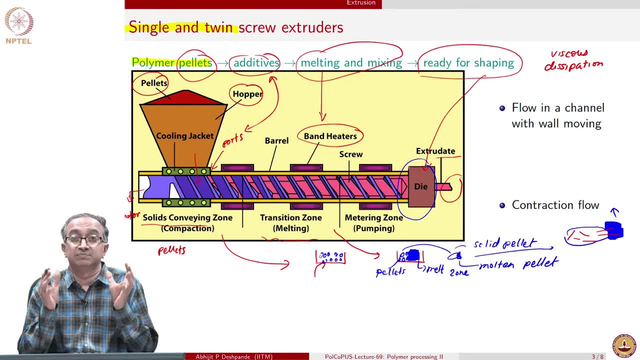 much narrower than the whatever is the barrel and the screw opening there because we force the material through a narrow die and do the shaping operation and finally get the extrudates. So you can see that, based on this description, the two classic problems of fluid mechanics. 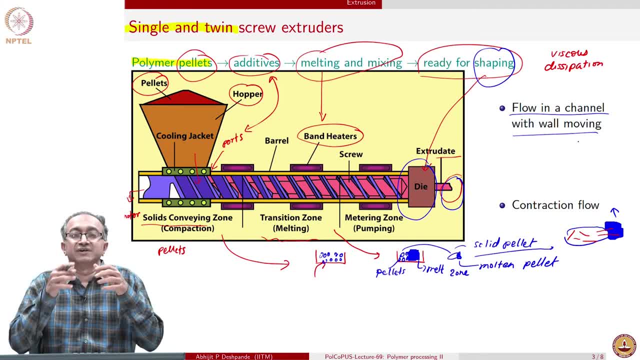 are flow in a chain, So this is where the screw is rotating and because of which polymer is also moving. So this is like saying that I have material between two plates and one plate is moving, because of which the polymer is also moving. 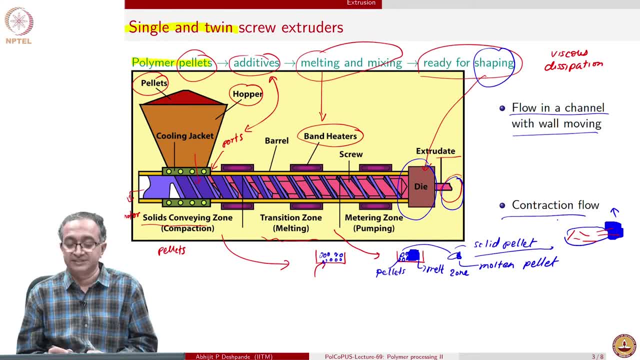 The other problem is that of a contraction, because we have basically polymer being pushed through a narrow opening so that we get the extrudate. And one of the important aspects of extrusion design is what is the shape of the extrudate and what is the shape of the die? 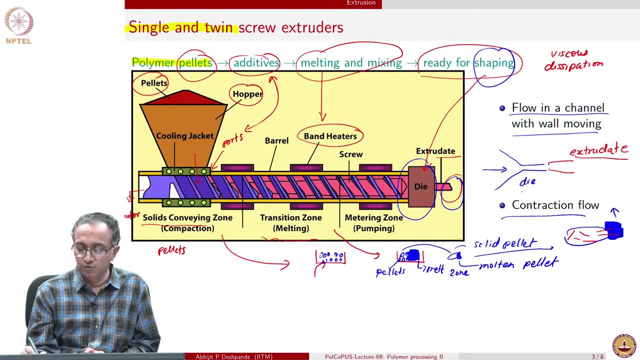 So the die opening shape and the extrudate shape, how are they related to each other? and that is an important part. We will see later on that extruded shape is not exactly the same as the die opening because of as soon as the polymer comes out, because of the elasticity, macromolecule were forced 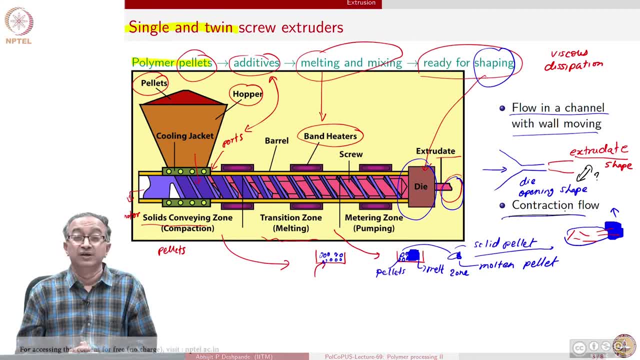 to go through a very narrow opening, And so contraction flow is very significantly influenced by the segmental mobility and the segmental flexibility that is there in the polymer. When we are forcing it to go through the narrow opening, the polymer molecules can get stretched. 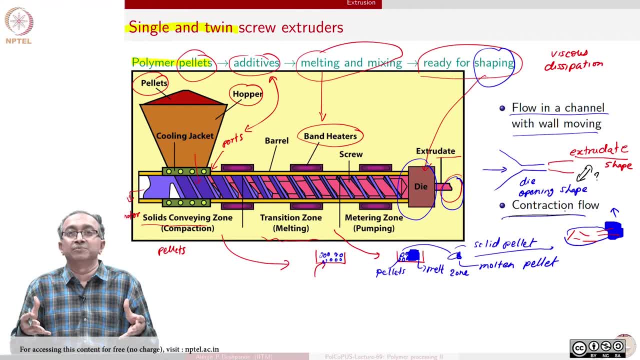 But as soon as it comes out, as soon as the extrudate is formed again, there is no opening there anymore and polymer segments can go back to their earlier conformation, And so this elasticity will induce a shape in extrudate which is different compared to. 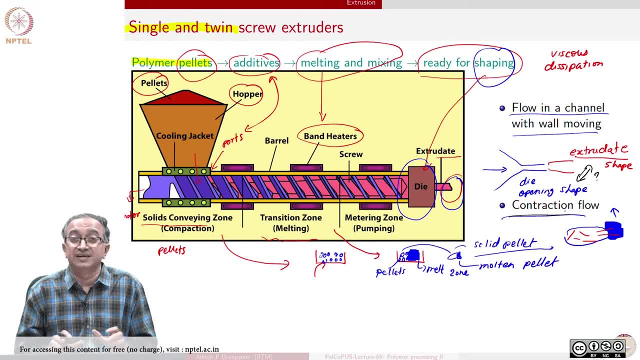 the opening. So you can see that an example process such as extrusion involves so many intricacies which are related to phase transfer, because solidification to melting is involved. then it involves flow And shaping and stretching and shear flow and extensional flow, flow through contraction. 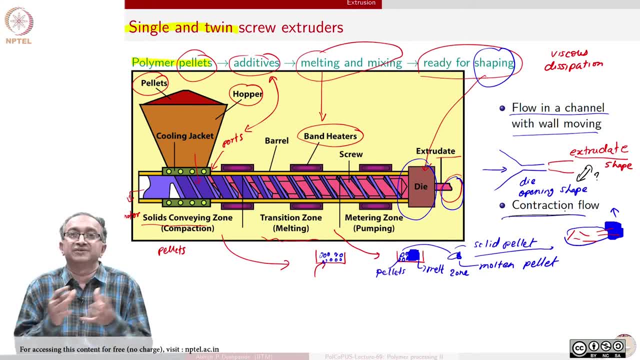 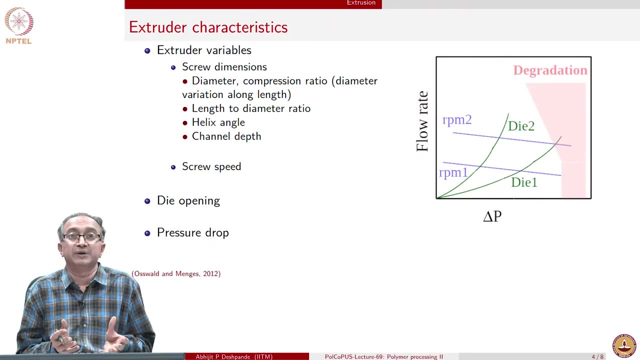 flow through a pipe, flow through a channel, so so many different examples are involved. And post extrusion, now the shaping can be done, you can stretch it again, and then finally cooling has to happen, solidification or crystallization, or vitrification, And so in this operation there are several parameters which are important. 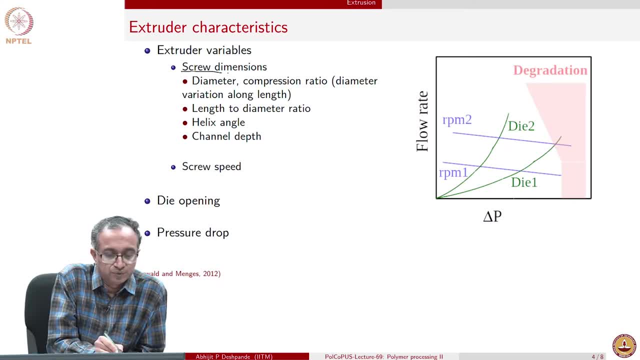 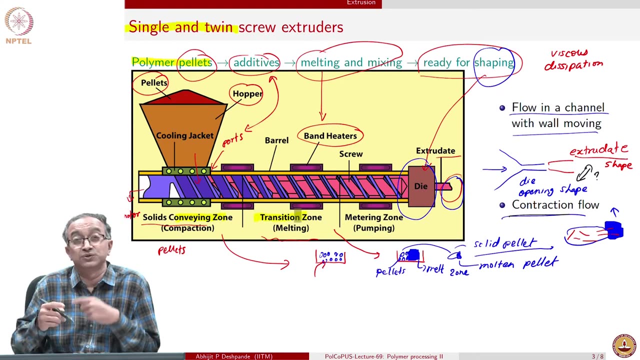 Based on the description that I gave. we already know that. you know screw dimensions will be very important: the diameter, the compression ratio. This compression ratio is important because that is what will determine how the conveying of solids happen and how does the transition zone melting happens. 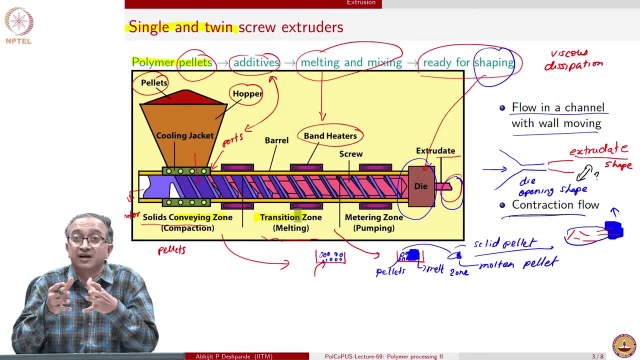 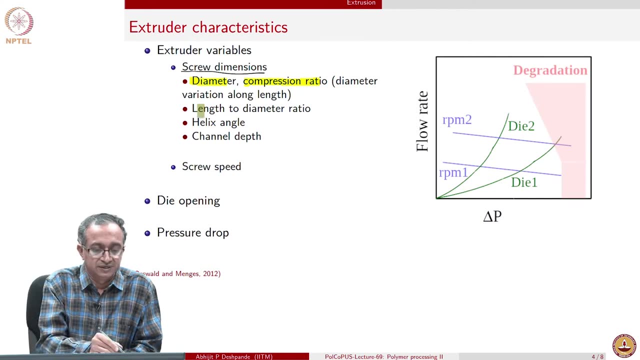 Because, basically, with this narrow opening becoming narrower, the solids get pushed and then, through viscous dissipation and the heating heaters which are there, we can have melting of the polymeric pellets. So therefore, compression ratio is important, the length to diameter ratio of the screw. 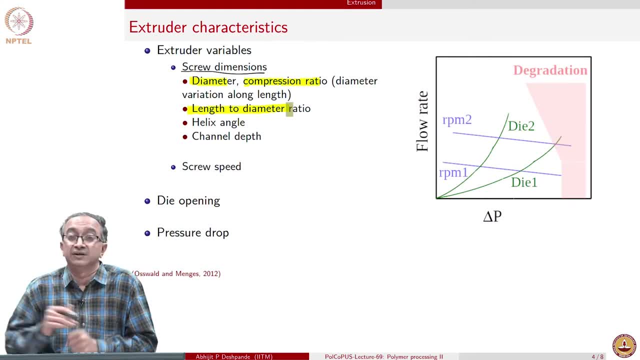 is important because that determines the how these different zones are separated from each other. The angle, that determines again how is the pumping action or the screw conveying action happening, and then the channel depth of course determines the overall amount of material that is available. Higher the channel depth, it also implies that the strain rate will be lower. and to explain, 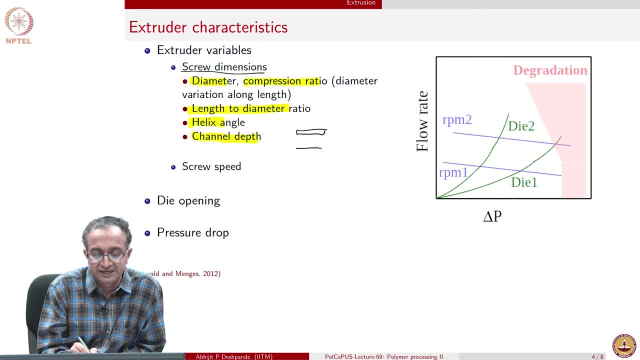 this. So think of this problem where, let us say, if I have a flat plate and I pull the top plate with certain velocity, there will be a certain strain rate in this. Now I take the same two plates, but now I have much narrower opening and I pull the. 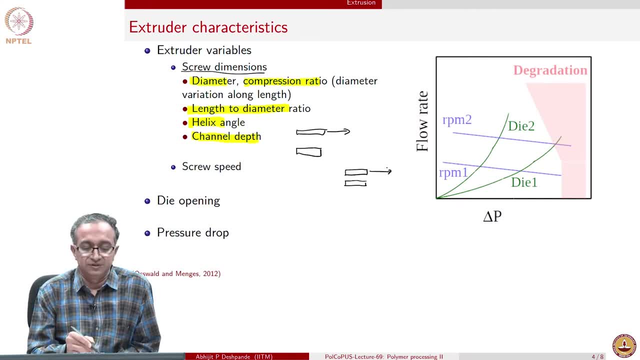 top plate with the same velocity. So this is equivalent to channel depth, because we could think of this as the screw moving at a given velocity. But if the channel depth is less, then the strain rate will be higher, because strain rate in all of these cases is the velocity of the screw divided by the channel depth. 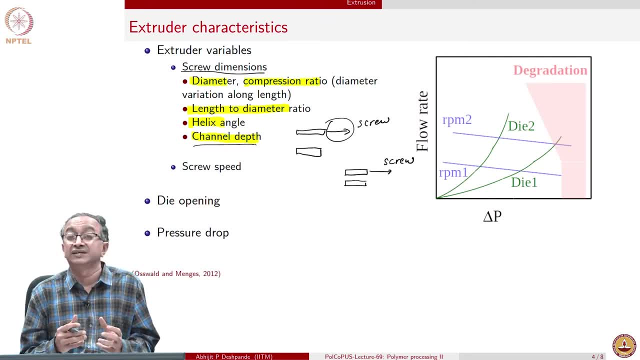 So, therefore, that determines the amount of strain rate, and we already know that strain rate influences the flow behavior of polymeric materials very significantly. And so screw speed and channel depth together, determine the strain rate in the material, Then finally the die opening and the overall pressure drop. 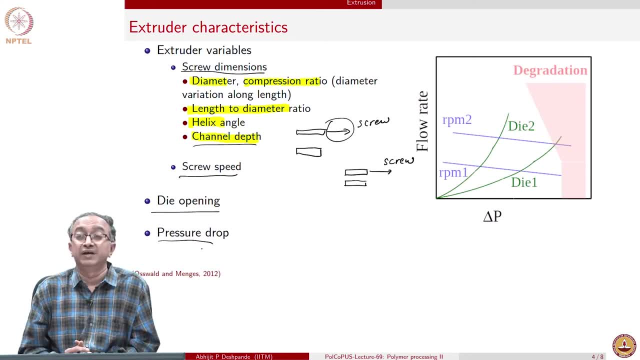 Because of pumping actions, determine what is the overall behavior of the extrusion operation and generally this can be shown using what is called an extruder characteristic. So we can look at flow rate, because we are interested in how much amount of polymer we can process per unit time. 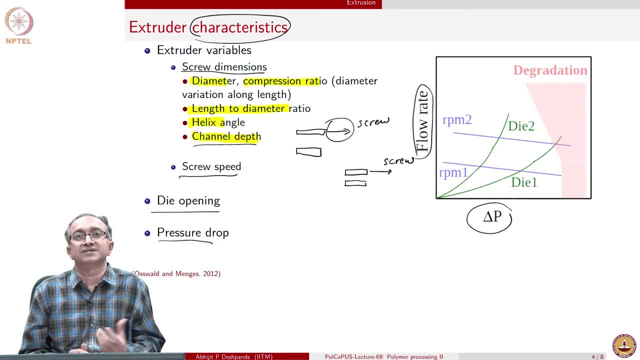 So that is, determine based on flow rate. We would like to make parts as fast as possible, and so, therefore, flow rate should be as high as possible. However, there are limitations. apply higher and higher pressure and again achieve this higher and higher flow rate. 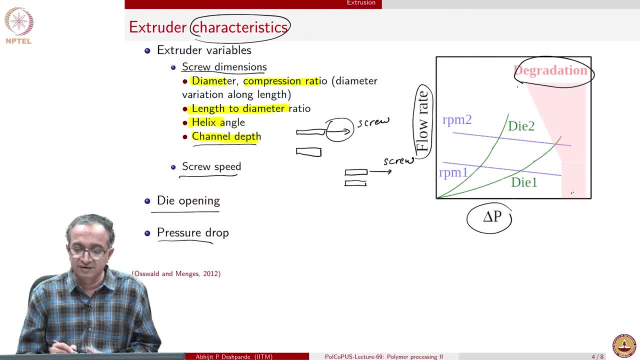 But when we go to extremely high pressure then and we will have degradation set in the material chain, scission and our reactions like that can degrade the polymer material. Now in this basically flow rate versus pressure drop can be thought of. when we think in fluid mechanics the standard problem we solve is pipe flow. 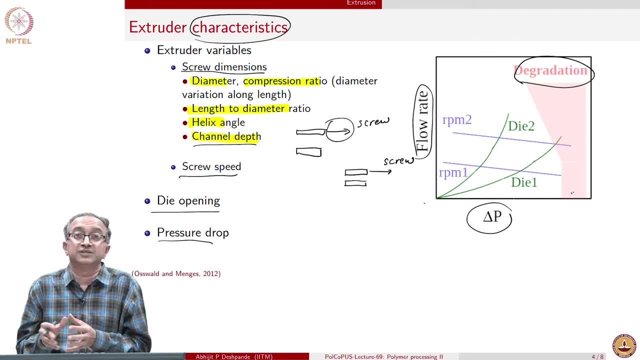 When in a pipe flow, if there is laminar flow, then we know that flow rate is proportional to pressure drop, So we will get a straight line. but here we have polymeric materials which are non-Newtonian as well, as we do not have a straightforward pipe, but the we have similar to a pipe whose 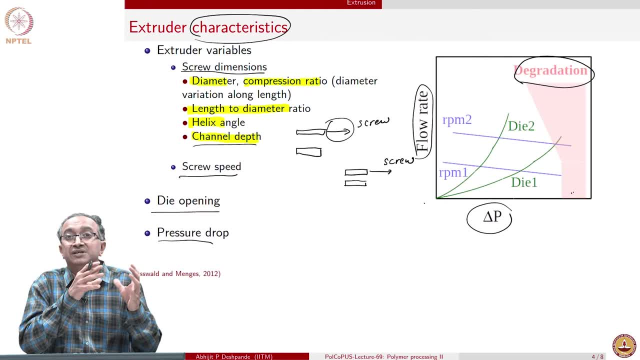 cross-sectional area keeps on decreasing because, remember, there is a compression ratio. So therefore, generally, pressure drop increasing will change the strain rate and therefore change the flow rate. So we can change the flow rate non-linearly, and this is the kind of behavior that you. 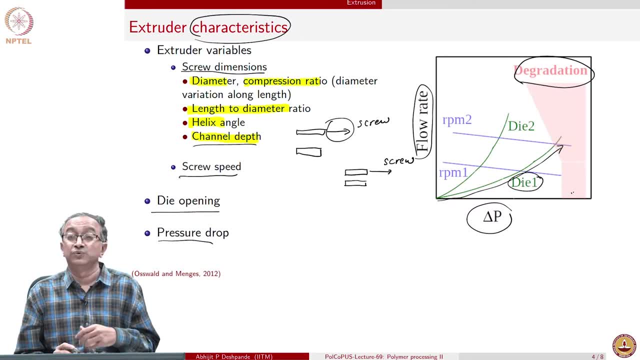 will obtain for one particular die. when you change the die size you will get a different flow rate versus pressure drop characteristic. Looking at this graph, can you make out which diameter of die is higher? is die 2 diameter high or die 1.. To think of it, you can just pose this question that at the same pressure drop which one gives 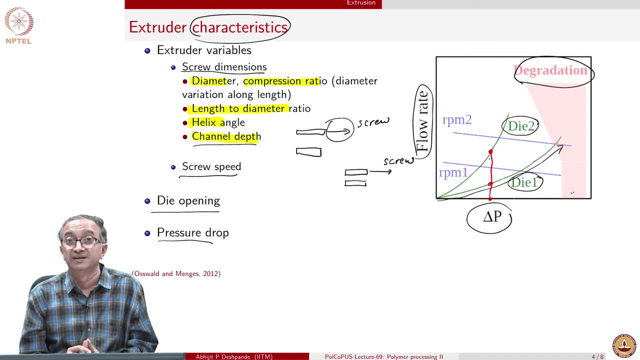 me higher flow rate and which one gives me lower flow rate and why So? I am sure then you can quickly see that die 2 ought to have a bigger opening, because I get much more flow rate from it, And similarly the screw speed also determines how much is the amount of material that I. 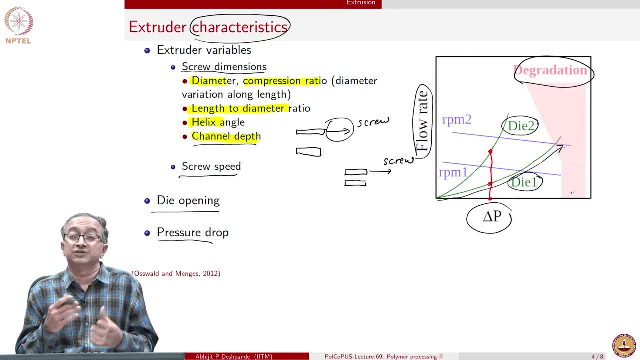 get and at different pressure drop. So at different pressure drops and screw speeds we will again have different characteristics. So generally this kind of a characteristic is drawn to each and every for every set of extruder system, and then we can decide which die to use, which rpm, to use how much delta. 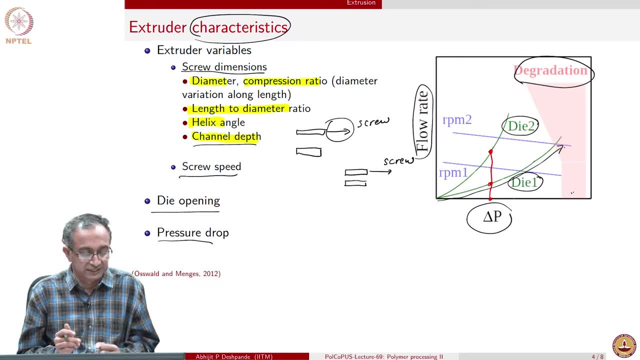 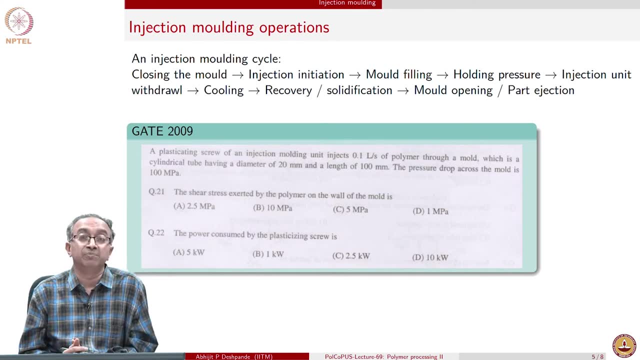 p to use and what kind of production rate will we get using the analysis of such characteristic curves? Let us shift and now look at the injection molding. Injection molding operations. injection molding is a cyclic process as opposed to the continuous process of extrusion, where we saw that melting happens and then it gets extruded and keeps. 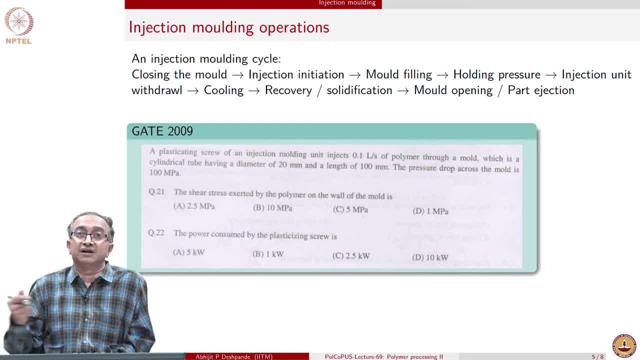 on getting pulled and then, therefore, it is a continuous operation. Injection molding, on the other hand, is a cyclic operation. How is it cyclic? What do we do? is we start with closing the mold? as soon as we close the mold, we imply that mold can be filled. 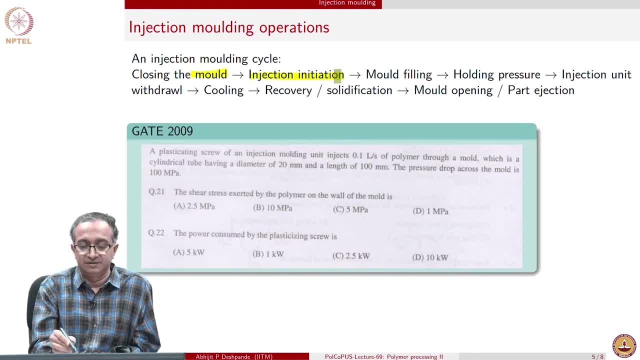 So therefore, then injection can be initiated. When we initiate the injection, mold filling happens, and then, once the mold is filled, we hold the material for some amount of time, and then we can withdraw the injection unit and simultaneously start cooling the sample so that recovery and solidification happens. 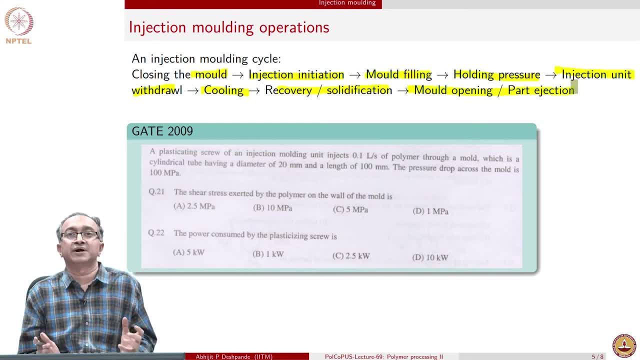 As soon as solidification happen, mold can be opened and part can be ejected. So this is nothing but again opening, and so the next stage again will be to close the mold. So it is a cycle which can continue, and strength of injection molding is all of this can be. 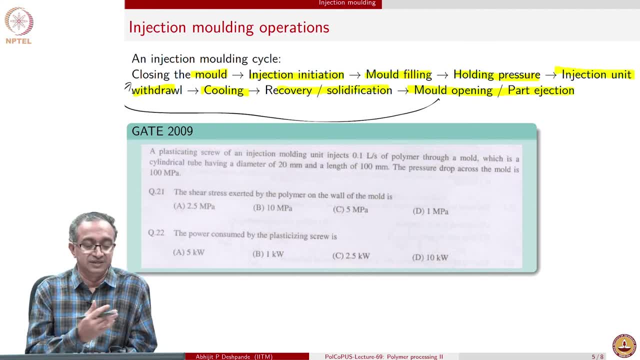 done in couple of seconds. that is how fast the injection molding processes. And the design of injection molding involves several calculations, again in terms of pressure drop and flow rate, and this exam question highlights that if you have an injection molding unit which delivers a certain amount of polymer and the dimensions of the, the tube in which 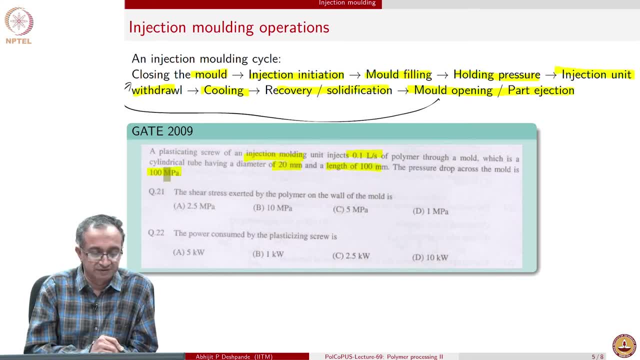 the delivery is happening is given and also pressure drop is given, then can we have an estimate of what is the amount of stress that is generated by this polymer, because the mold itself is not moving. So what will be the amount of pressure, that is, stress that is generated, and then whatever? 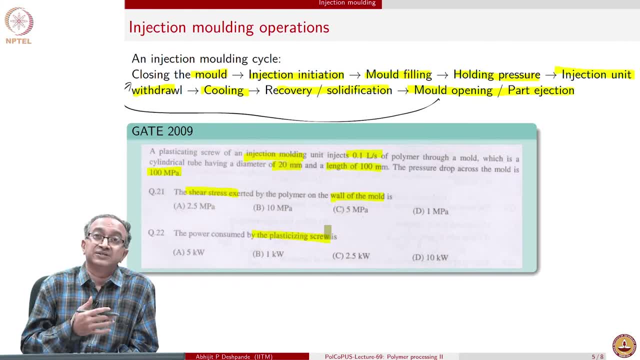 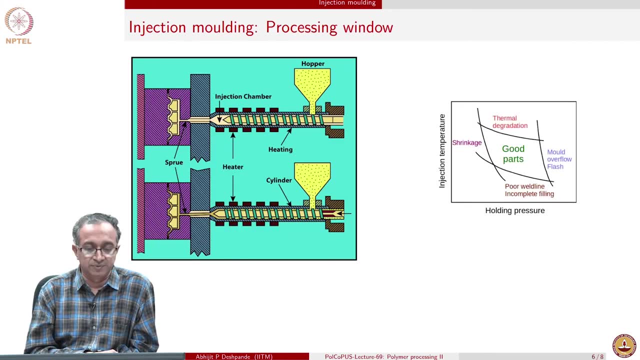 is the amount of power that is required for the screw to actually convey the material to the molds. So you can think about this while we discuss the injection processing operation In little more detail. so initial part of the operation again looks like the extrusion. 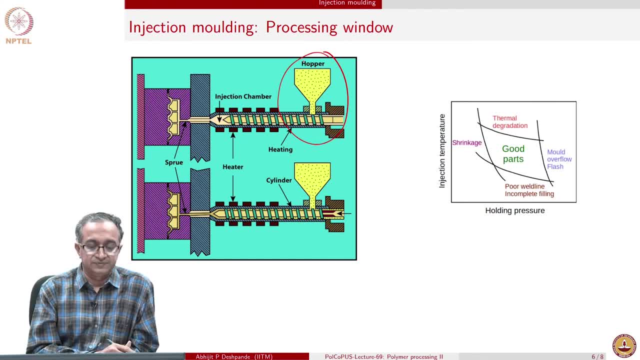 where, through a hopper, pellets are fed. In this case, though, we already have a set of pellets which are mixed, So the role in this case of the injection unit is to just make the polymer into a molten form so that it can be delivered to the molds. 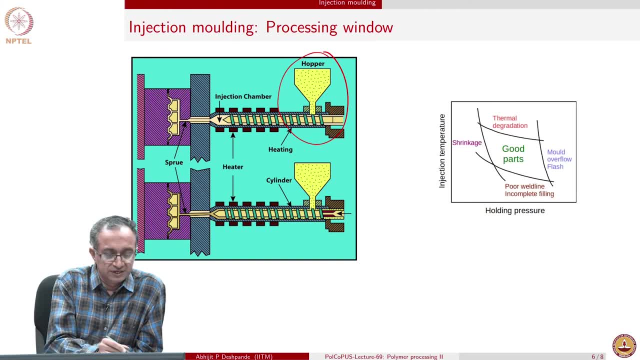 And in as soon as the mold is closed. Then what we have is there is an injection chamber in which fluid will accumulate and then, when the screw moves forward, the injection material can then flow and then fill the gap. So you can see here that the mold is empty. 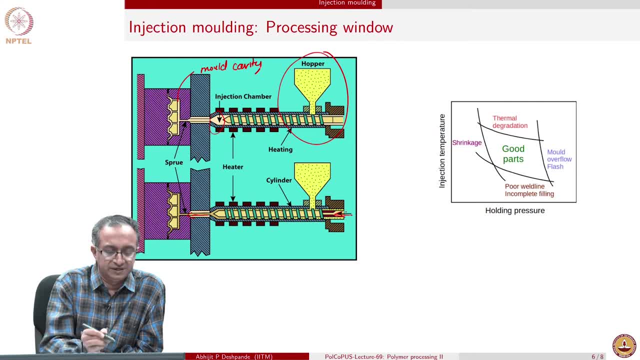 This is the mold cavity, so to speak, in which the fluid has to come and flow. So mold filling is happening And again, to melt, the polymer heaters will be there And the barrel. So the ventricle barrel is there and then there is again a narrow opening through which 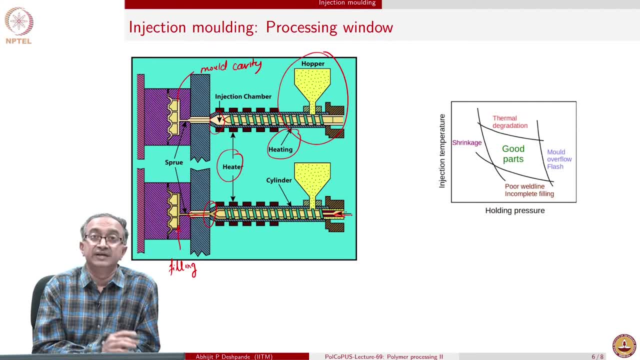 the polymer will have to flow and then flow into the mold. In this case, what is? the complexity of shape in the mold itself is also very important, And for toys or various other things the shape can be very complex. In certain section, the part can be very thin. some other section, the part can be very thick. 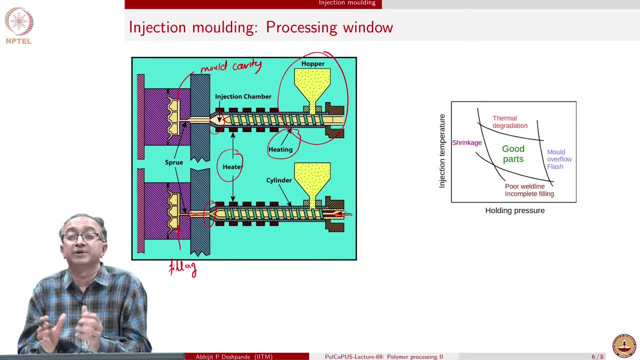 And so all of this flow has to happen, and again there is an operating window, And that operating window can be thought of in terms of pressure and temperature. If we change the temperature of molding, then the viscosity will be lower. flow behavior may be easy. 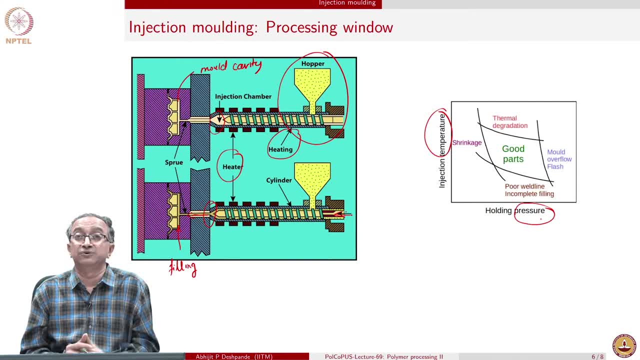 And similarly, by applying higher pressure we may be able to quickly do the process. However, there are again limitations. if we have too high a temperature, then thermal degradation can take place. If we apply too much of pressure, then the mold can overflow. Remember that. 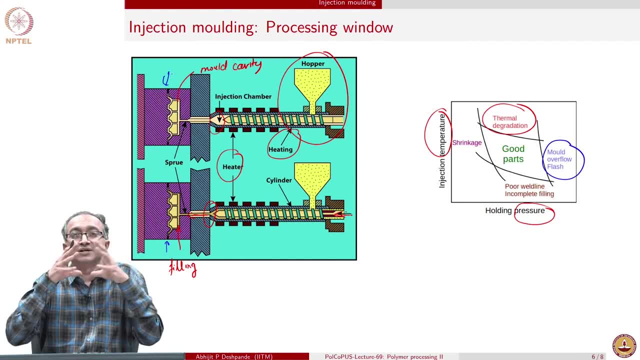 there is always this mold closing and the two parts of the mold are coming and closing. If you apply too much of a pressure, then there will be narrow openings in which the mold has closed. material will starts flowing. So there will be what is called a flash, which implies polymer coming out of the mold, which 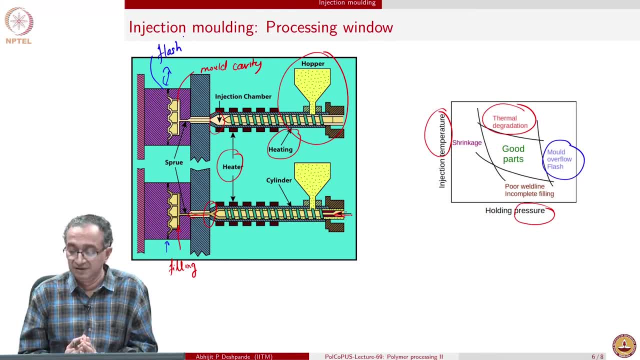 is closed, but it cannot be ensured that it is completely sealed or leak proof. On the other hand, if you apply less temperature, then what happens is the polymer segmental mobility and macromolecular motion is not very fast. and when polymer comes in contact, 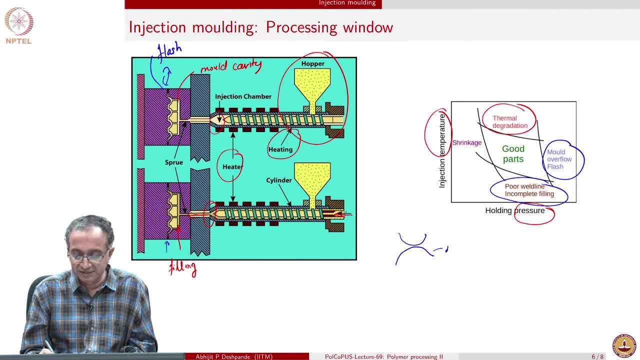 with another polymer melt. so this is, let us say, melt front and this is also melt front, and when they come in combined contact with each other. So the macromolecular segment from this and macromolecular segment from this should intermingle for you to get a good weld line. 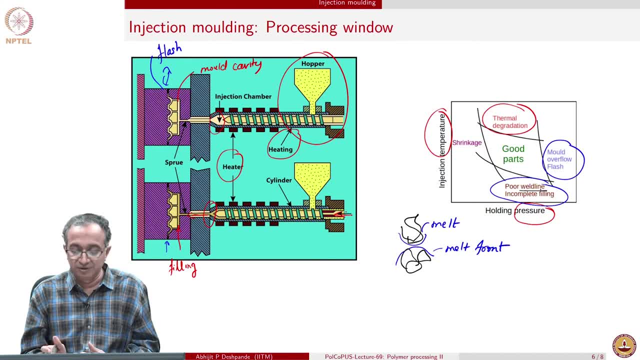 In fact, no weld line will imply that there is perfect mixing. but at low temperature what happens is macromolecular flexibility is less and therefore we get a weld line which is quite prominent and that becomes basically the weak spot. or sometimes the viscosity can be so high that the filling is incomplete. 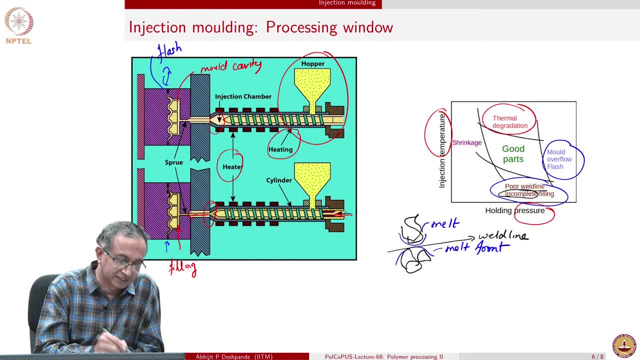 So you know, some places the polymer does not reach, and in that case we will have incomplete filling, So the filling process itself is not very efficient. So again, low temperature is not desirable. If we maintain too low a pressure, then again there, once the part comes out, there will be. 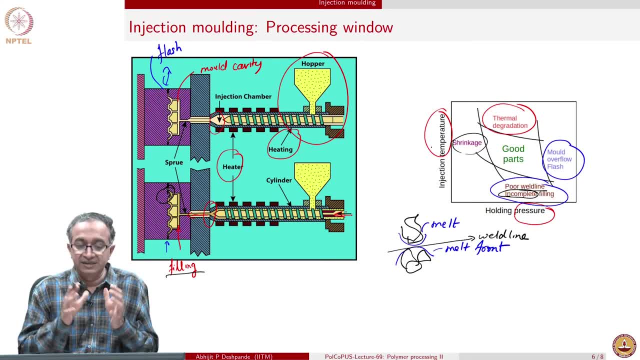 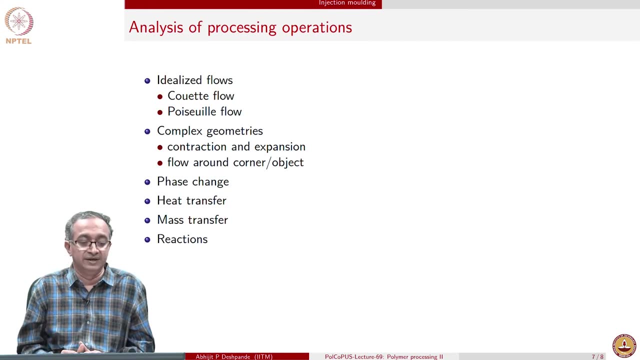 significant amount of shrinkage, because maintaining pressure and allowing stabilization of the overall polymeric material is important. So with this, we have seen two important processing operations- extrusion and injection molding- and we have seen how flow is very important and therefore analysis of these. 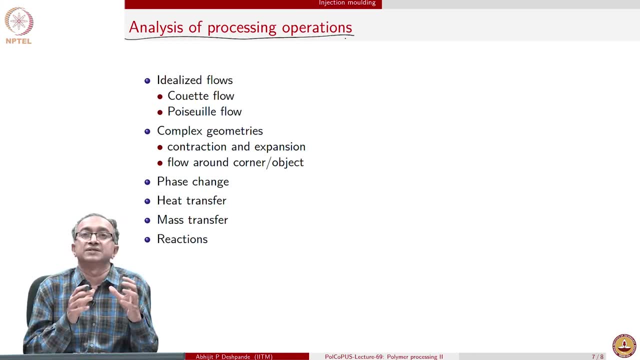 processing operations in terms of flow. behavior involves some of these features. We look at flow in an idealized sense. We look at a Couette flow, which basically implies taking the material between a moving solid surface. So this is Couette flow. We could also look at Poiseuille flow, in which case we have a cylindrical pipe and then we 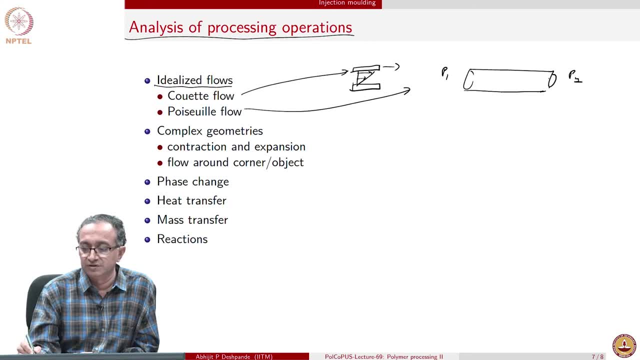 impose a pressure gradient and force the polymer to flow through this, and in this case, of course, we may get a velocity profile where it is maximum at the center and 0 at the surfaces. So these are two ideal types of flows and you can see, both of these are important when 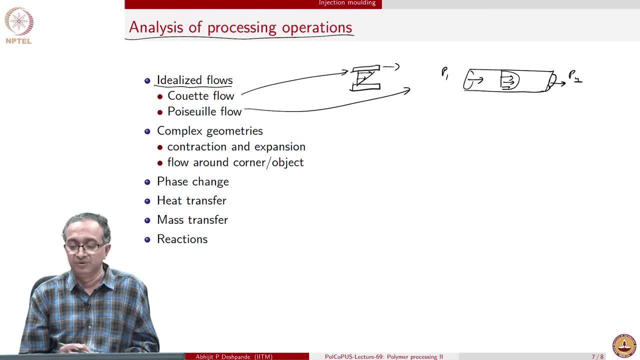 extruder screw is moving, then we have a Couette flow. So if we have the pumping operation, in which pump is it is creating pressure, then we have Poiseuille flow because extrusion die when the material is coming out. pressure is very 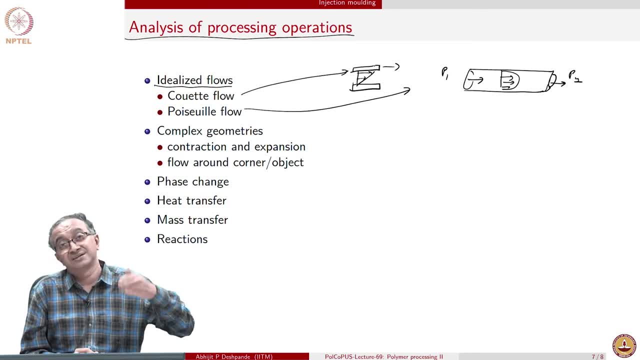 high in the extruder because we have all this screw, action and fluid is basically being forced to move and therefore pressure is extremely high. and the other side, it is atmospheric pressure, because that is the extrudate where the polymer has come out, and so we have a. 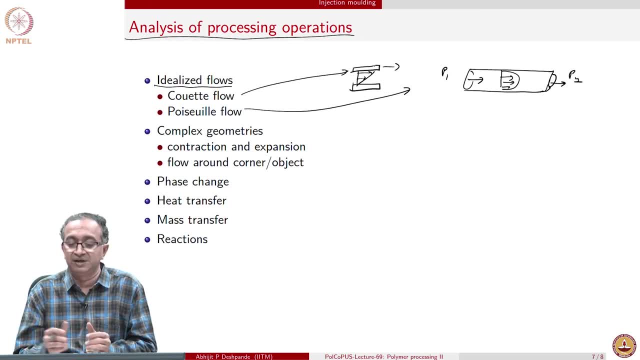 pressure gradient and so flow through the die opening. It can be analyzed using Poiseuille flow and of course we have complex geometries. So there is contraction and expansion, because as soon as the material comes out in the mold it is like expansion, but it is going through the extrusion die. then there is contraction. 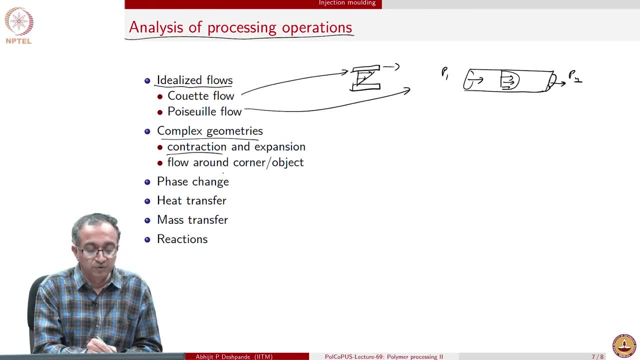 So both contraction and expansion flows are involved, flow around corners and objects are involved. we can have an opening, like this contraction, where fluid is flowing, and we can have these corners And the flow around corner may be very different. in fact, there may be a stagnation zone where 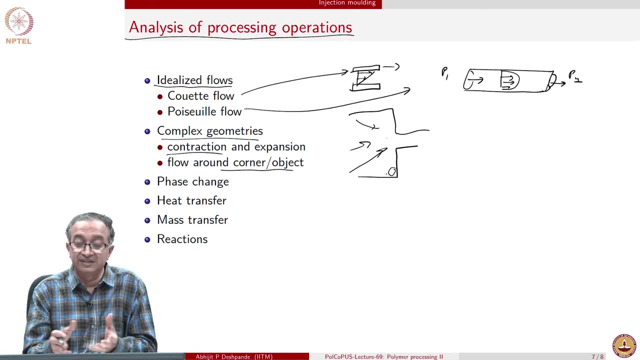 polymer may start solidifying or degrading and once in a while that polymer joins the flow and therefore it comes out that will compromise the performance of the part. So all of these complex geometry flows are very important. additionally, we have solid to liquid phase transition. if there are some volatiles in case of foaming operations, we 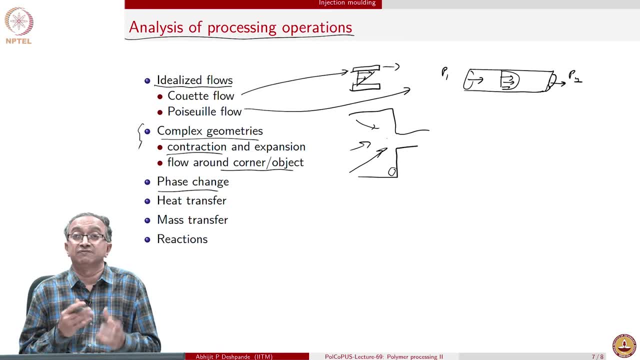 will definitely have blowing agents And whenever there is phase change, there also heating and cooling are important part in terms of melting as well as solidification. and if, let us say, crystallization or polymerization are happening simultaneously, those bring in heat release. whenever there is polymerization, 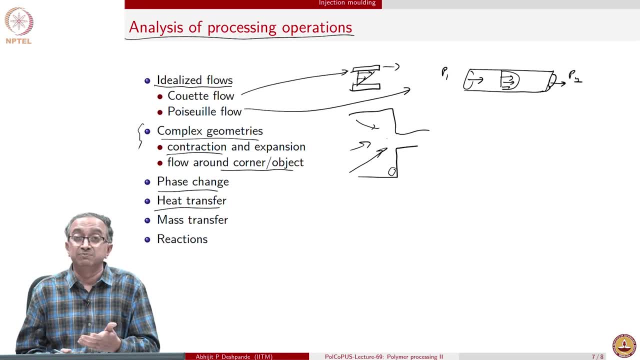 happening, heat absorption if there is melting happening. So all of these involve basically transfer of heat. and then we have mixing and mixing of space. We have mixing of small molecules with macromolecules, mixing of one macromolecule with another macromolecule. 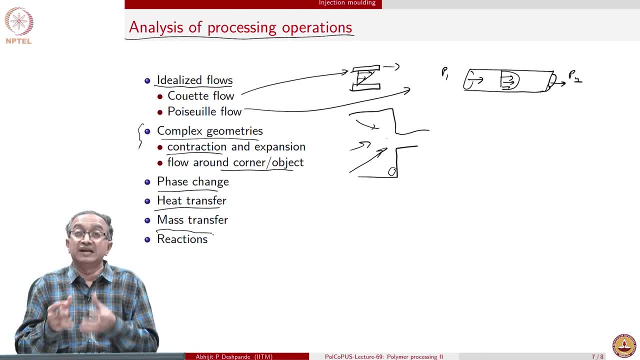 mixing of the same macromolecule in a mold where weld lines can be formed. So mass transfer is also extremely important. and finally, of course, we can have reactions. So if we have to analyze processing operations, these are all the features which need to be.